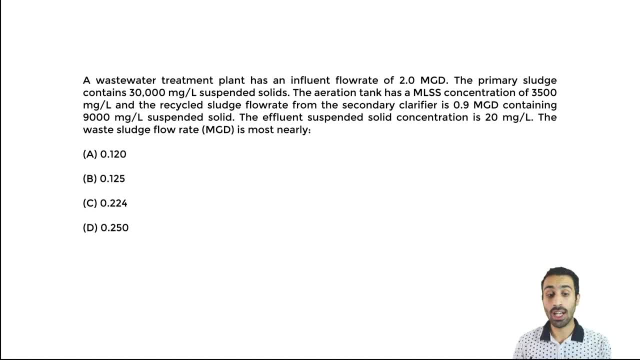 It's OK if you get stuck. It's OK if you make mistakes, because I know when I did this the first time I did make a mistake. Now I've learned from that and I'm going to redo it with you to show you. 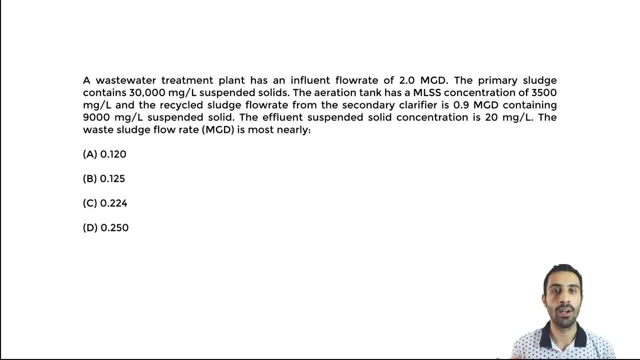 These right steps to arrive at that final answer. So please pause the video. struggle through it. It's OK if you get stuck. This is not an easy one and it can be a little tricky, especially for activated sludge and wastewater treatment. 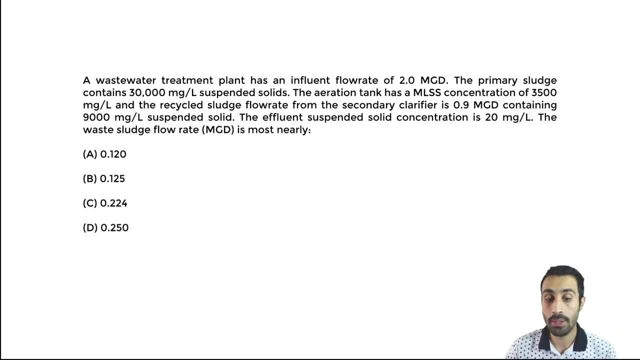 OK, let's read this problem statement. We're told a wastewater treatment plant has an influent flow rate of two MGD million gallon per day. So in the US this is the units like for water, wastewater treatment. We have these usually in million gallon per day. 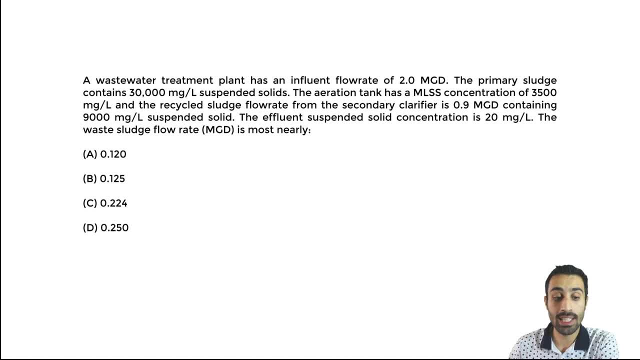 Those are the common units. The primary sludge contains 30,000 milligram per liter of suspended solids, The aeration tank has a MLSS mixed liquor suspended solids concentration of 3,500 milligram per liter, And the recycled sludge flow rate from the secondary clarifier is 0.9 MGD, containing 9,000 milligram per liter suspended solids. 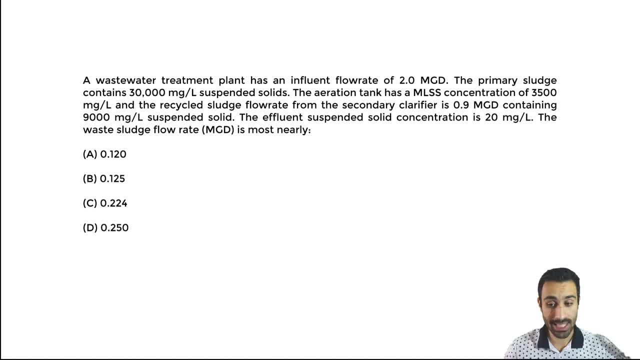 So that's a long sentence there. This is saying: MLSS is this concentration and the recycled sludge flow rate. We know we always recycle that sludge that has this flow rate. Q recycled is 0.9 MGD but it has a concentration of 9,000 milligram per liter. 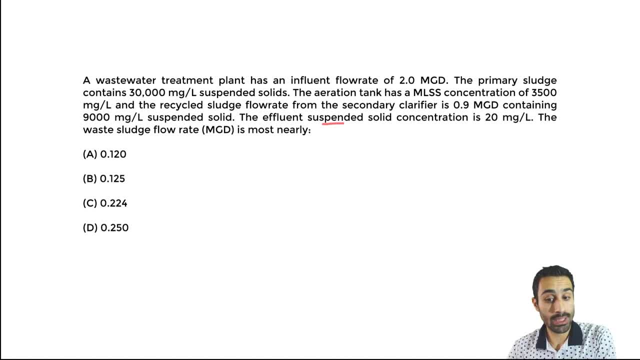 And we'll denote that on a diagram as well. The effluent suspended solids concentration is 20 milligram per liter. So the effluent is like what The effluent comes out after secondary treatment at the final, in the final stages of the treatment train. 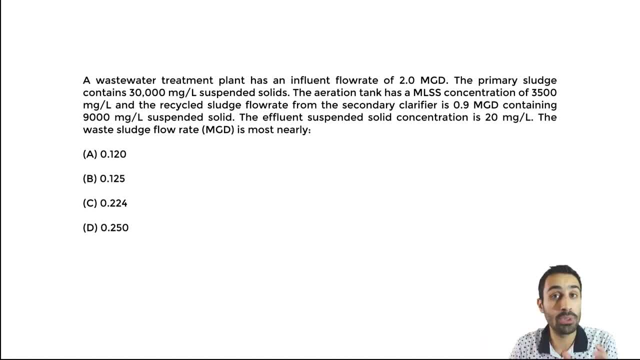 So we're told the waste sludge flow rate in MGD is most nearly what. So first let me do know what I want to find. I want to find the waste sludge flow rate, and we can denote it as QW, And that's how it's denoted in the handbook. 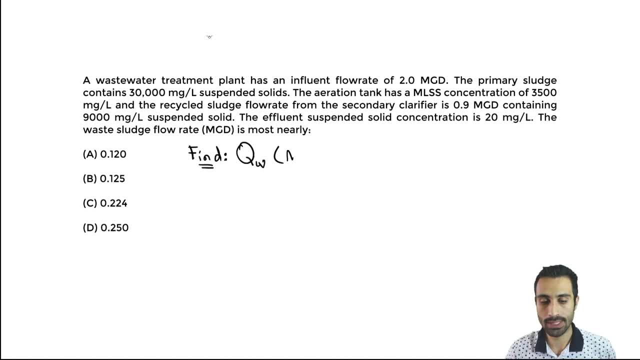 And let me write it as QW- And we want units in MGD. So we know In this case everything will be MGD, So we don't really have to worry about the units. But what I'll show us at the end is how to convert it to gallons per day, because right now it's million gallon per day. 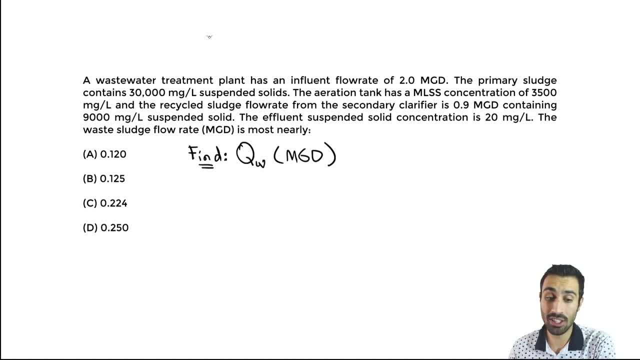 So this is what we want to find, And what we can do next is actually begin denoting what we're given. So let's draw what we're given, And what we can do first is actually draw the system, draw this overall treatment. 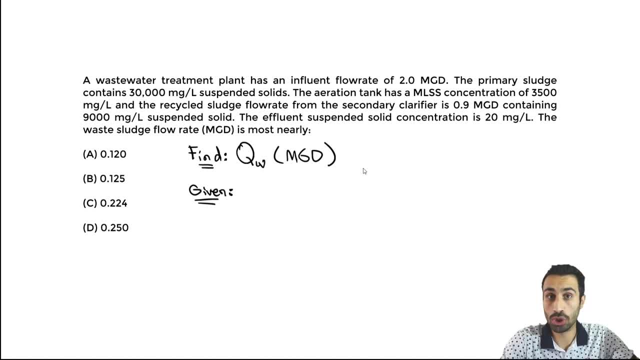 And the most important part in this case is that biological treatment, Which we call secondary treatment. That's where we're going to focus on in this one, especially because they ask us to find QW. We know QW occurs in secondary treatment, where we have the aeration tank and the secondary clarifier. 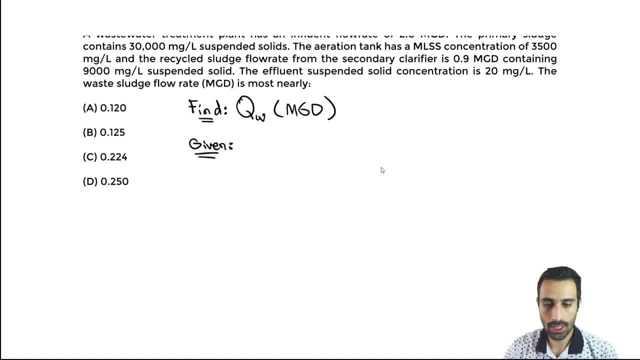 Secondary treatment is that system. So what I can do first is actually denote my primary clarifier. So in this case I'll just use a circle and call it the primary Primary, And you can think of it as the primary sedimentation basin. 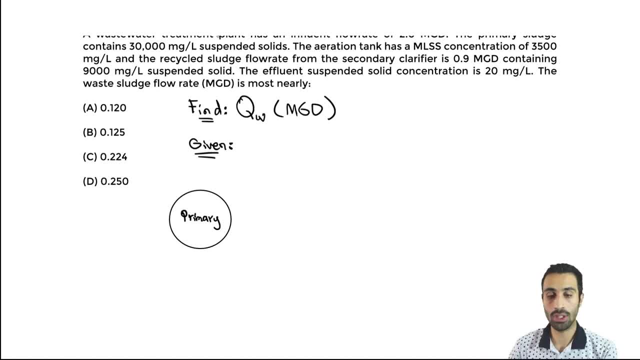 So what comes after primary? The aeration tank. So we'll put the aeration tank right after that And I can denote it like this: And we know this is going to be my aeration tank And this will always have volume as well. 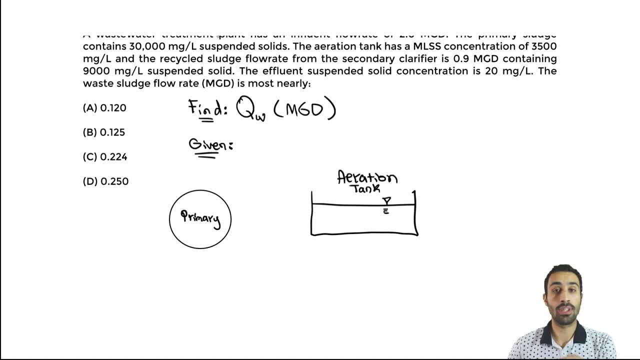 So aeration tank, And after the aeration tank, what comes? Secondary, Secondary, Secondary, Secondary. It's the secondary clarifier, which is like a secondary sedimentation basin. So just know, clarifier means sedimentation basin. Same thing. 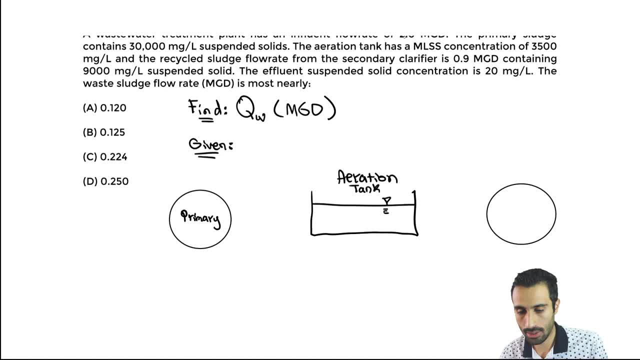 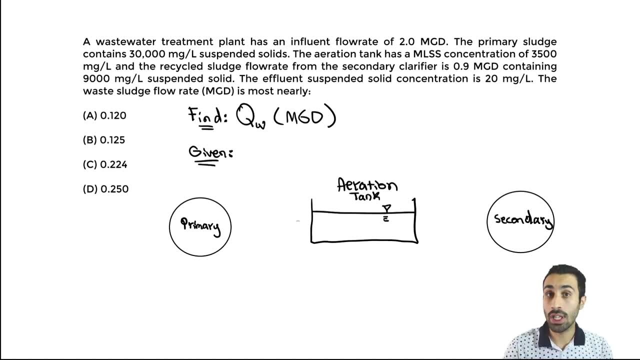 So now it's, this will be my secondary, and I'll denote it as a circle as well, And I'll call it secondary. Now let's start putting the numbers that were given on our diagram. So first of all, we're told the wastewater treatment plant has an influent flow rate of 2 MGD. 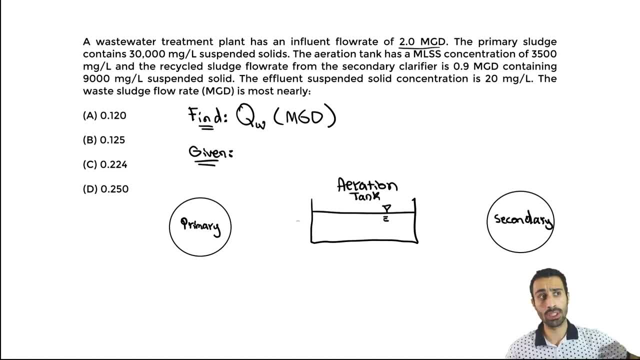 I'm going to put that as what comes in into the plant, So we know it comes in. We have the great chambers. We have the screens great chamber, maybe an equalization basin. Then we have that primary, but that flow is just going to stay at 2 MGD when it enters the primary. 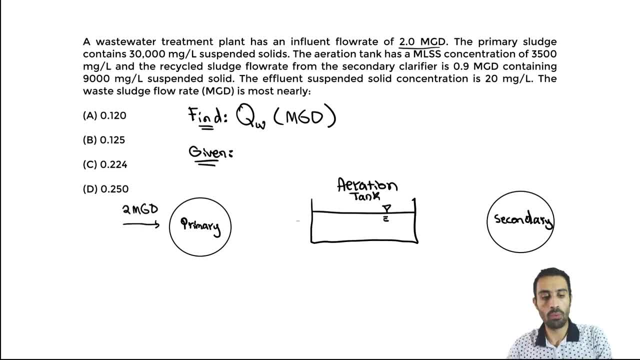 So it's 2 MGD. So I want to know the primary actually does have some sludge that comes out. at the bottom It's like a sedimentation basin and we have some settling and at the bottom we do have some sludge. 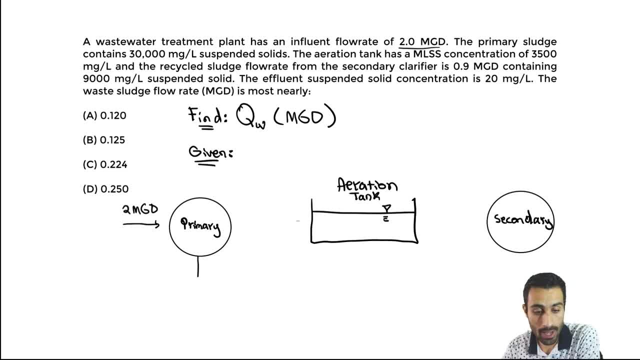 That comes out. So what I can denote and be accurate here is say we do have some sludge that's wasted from that primary and it does come out at the flow rate. But that flow rate is usually so small that the 2 MGD will come in and come out. 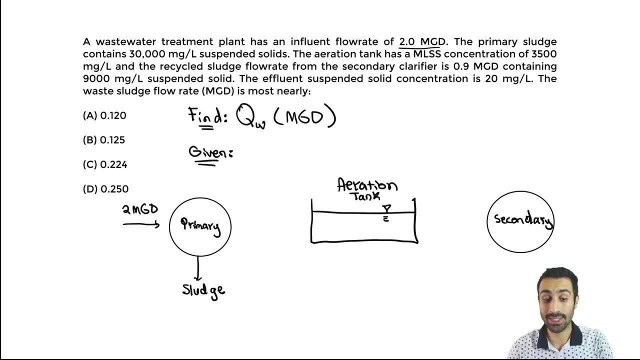 So we're not going to really apply a mass balance around that primary to get what comes out in terms of the flow rate. We're going to say that 2 MGD Of that comes in into the whole wastewater plant. is what is going to be coming in and coming out the primary. 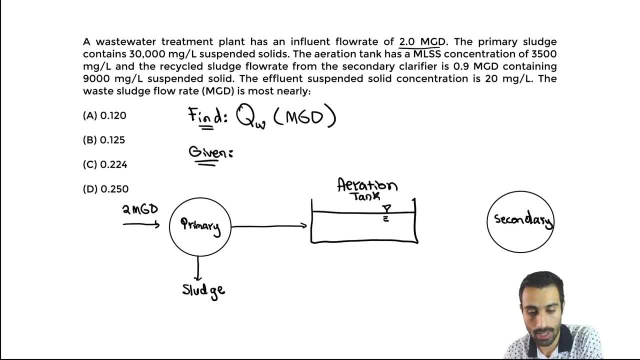 So in this case we can denote it coming out like this: Then it goes into the aeration tank and I can put 2 MGD here For that. So then, what else are we given? We're told the primary sludge contains 30,000 milligram per liter of suspended solids. 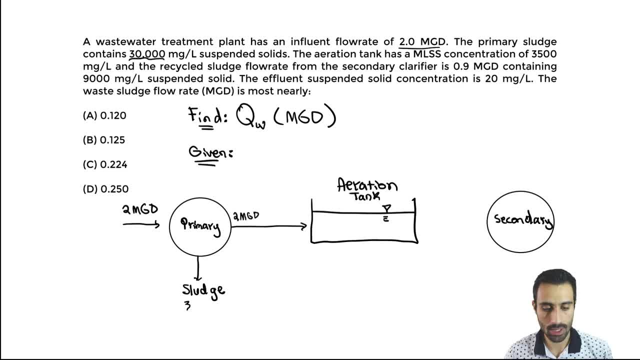 So we will say, okay, this will have a suspended solids of 30,000. Milligram per liter. but we will see this is actually not relevant and not important to solve this practice question. And maybe if we were trying to find the total sludge that's wasted for the primary and secondary, maybe that's a question, but in this one it's not going to be relevant and it's not important to solve the question. 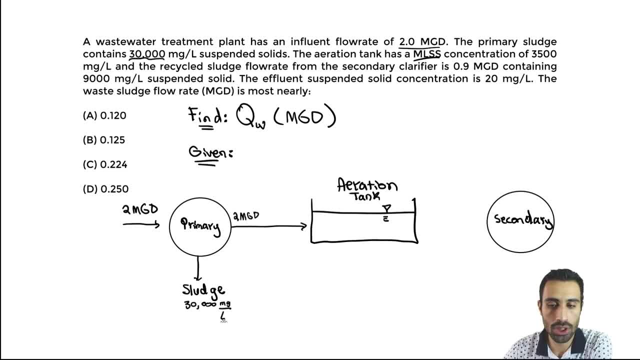 So then we're told the aeration tank has a MLSS concentration of 3,500 milligram per liter. So I can denote that as X or XA. I'm going to stick with the FE handbook and call it XA. and no MLSS is always in the aeration tank. 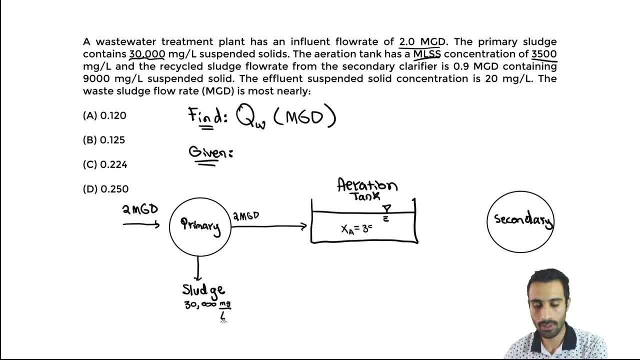 So that's going to be 3,500.. So we call that in milligram per liter mixed liquor suspended solids. So if you see X or XA, usually it's that it will be that in the aeration tank. So from there we're told the recycled sludge flow rate is 0.9.. 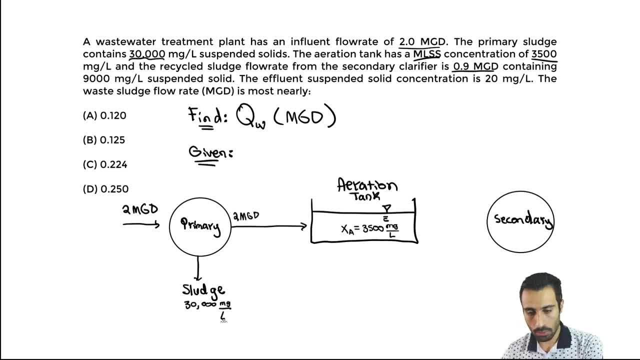 So now we want to know that this comes in and we have some flow that comes out and we know from the secondary we do recycle some flow and it goes back and we will go in. here We're recycling this. So this will have a QR value and that QR will be the 0.9 MGD. 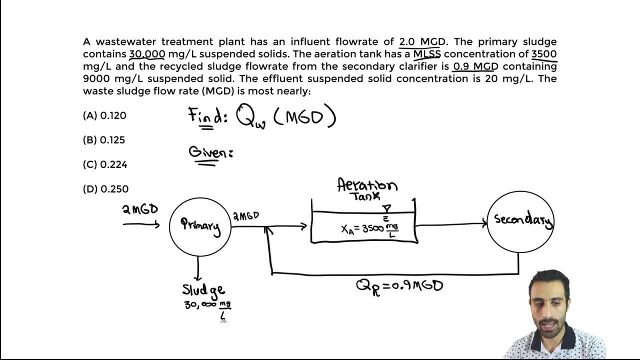 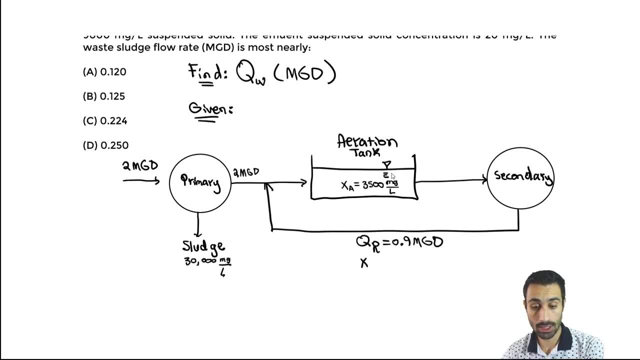 So that's that and that's what's given, And it contains 9,000.. Milligram per liter. So when they say 9,000, they're referring to the X or it's the suspended solid concentration: 9,000 milligram per liter. 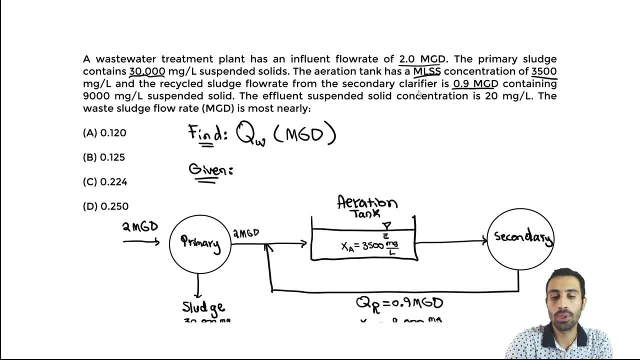 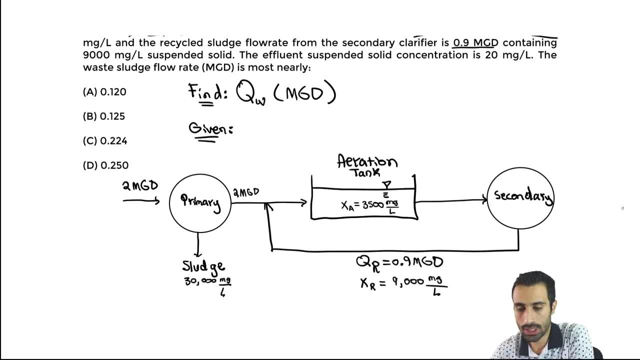 So that is denoted, Then we can keep going. It says: the affluent suspended solids is 20 milligrams per liter. That's what comes out the secondary. So we will say: affluent is always at the very end After secondary and we denote that. 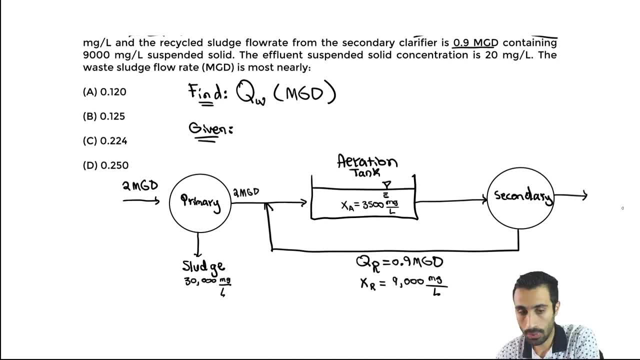 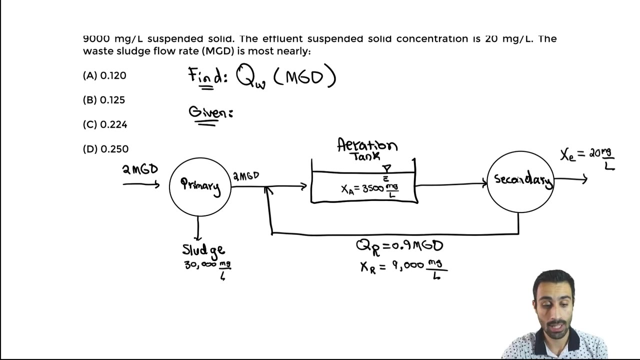 As. so the concentration is going to be X. So we can denote that as X effluent, E for effluent as 20 milligram per liter. And then we want to find Q waste in MGD. So now my question for you is: where's Q waste? Q waste is going to get wasted from the secondary 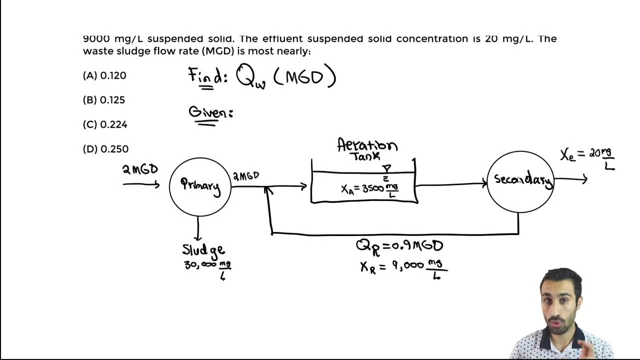 Yes, we do waste from the primary, But usually what we're focused on for that secondary treatment, for something like the FE, is that QW, which is going to be This. we can show it like this: QW is the question here, And when you have a QW, we do have a XW. XW, which is the suspended solid concentration of the wasted sludge. 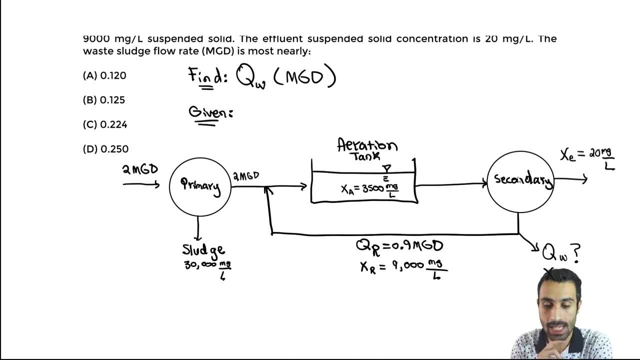 So now, what is that going to be? We can get that. We know it gets recycled at XR. Would you agree with me that XR is XW? It is, it's the same concentration. So XW is actually XR, So it should be 9000, even though that's not stated. 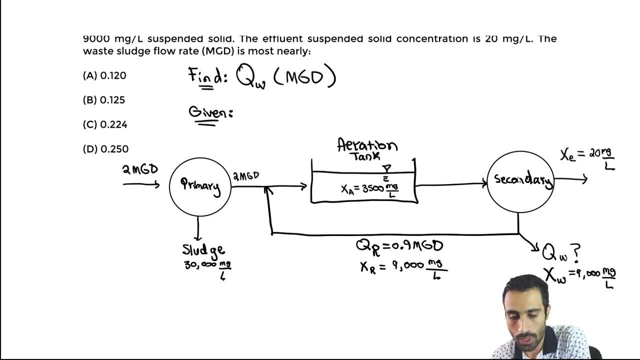 That's something we have to know. milligram per liter. So XW is always going to be the same as XR, and from there we can break this down a little bit more. But before that I just want to Use the FE handbook just to expose us to that. 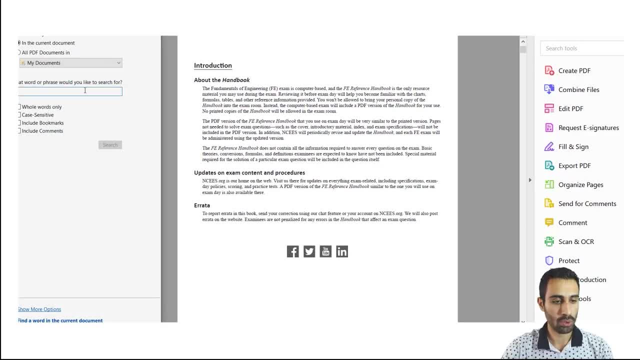 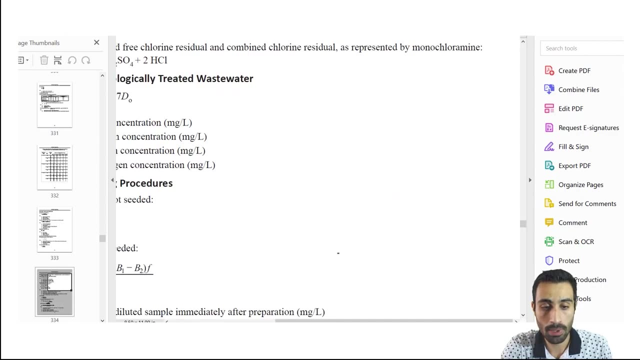 So if I go in the handbook, I can do the control, shift F and type, in this case, activated sludge, or you can type activate it and it's going to give you that page. and that's going to be the most important section, And what we will focus on in this case is actually going to be the value for this steady state mass balance. 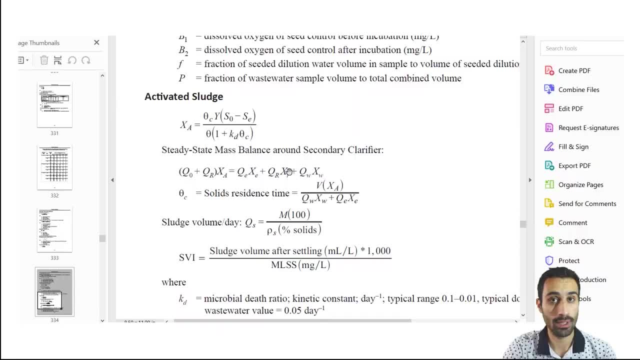 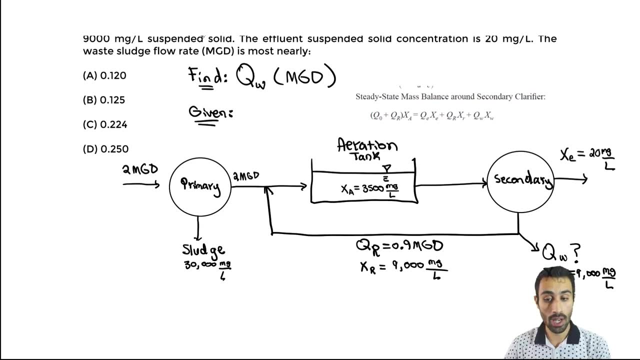 So we're going to apply this equation to solve this question. So I brought in the equation for us and we know we're going to apply this around a mass balance for the secondary clarifier. So what they're doing here is essentially looking at a mass balance around this part, which is actually what we need. 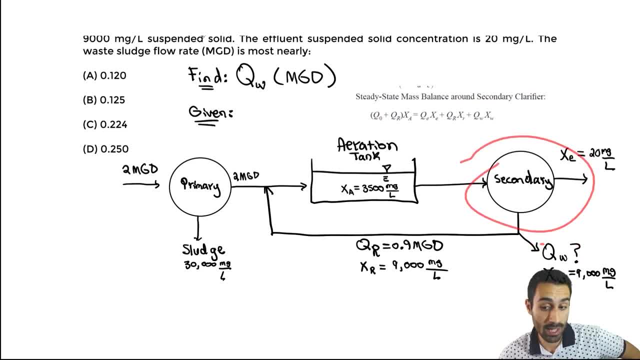 This is what we need to find QW. It's a mass balance. Think of a control volume around that secondary clarifier is what they're showing. It's not the whole treatment train. that's different. So we can have a control volume about this. 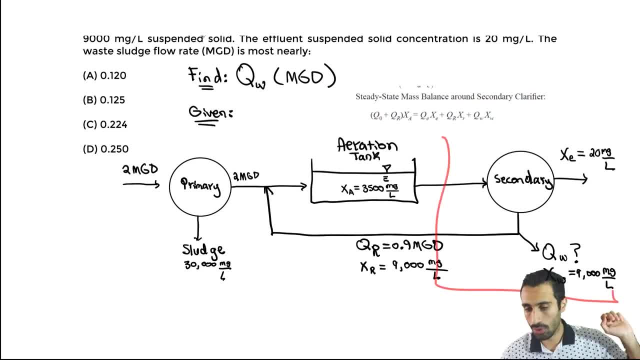 That's different A control volume about this. This one shows a control volume about the secondary clarifier. So now we know that this Q naught plus QR is something we did not denote here. So this is actually what comes in to secondary treatment. 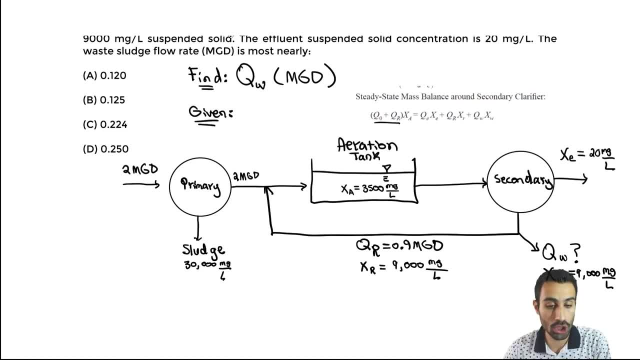 This whole process here is secondary treatment. Q naught plus QR will be the QR that gets recycled. Then it comes in to the whole secondary treatment and that Q naught And QR is what comes out the aeration tank. So what I can do for us. 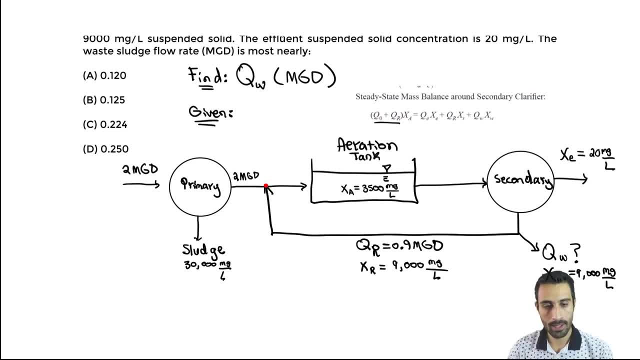 I want to be careful here. Let me put this point here. Then what happens right after that point is we have the Q naught Plus QR And this Q naught plus QR is going to be this Q naught. This is actually our Q naught, and think of that as that effluent out of the primary tank. 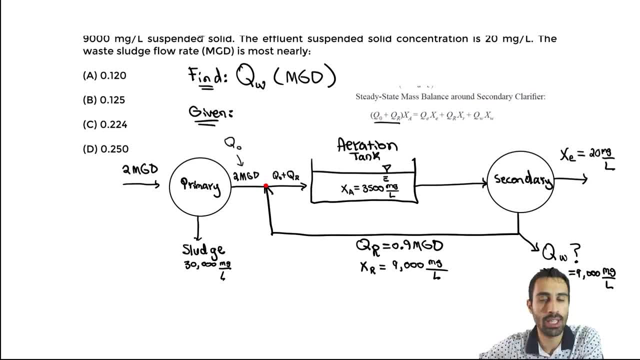 Which is the influence into the aeration tank and overall secondary treatment. So that's going to be the Q naught, This is Q naught. So then we go back, we can apply continuity or like what comes in has to come out around this point. 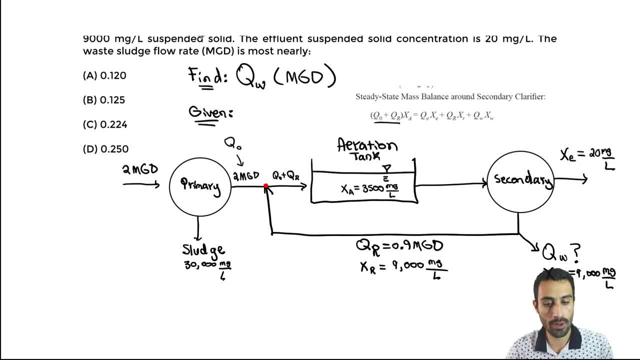 And then what comes out here will be Q naught plus QR into this whole portion. So that's Q naught plus QR. and this same Q naught plus QR goes into the aeration tank and it has to come out. So it's actually the same as this Q naught plus QR that comes out the tank and that Q naught plus QR will have a concentration. 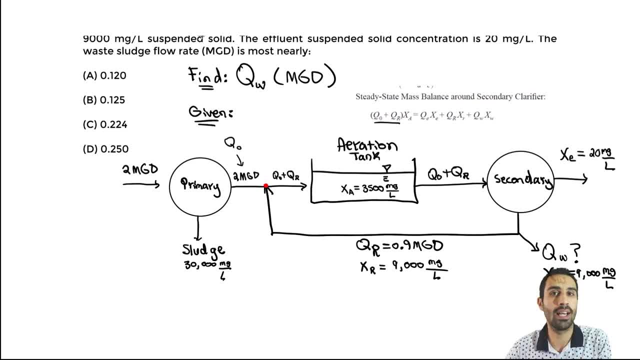 They denote that as X8.. It's the concentration MLSS from the tank. So it brings with it that concentration X8 from the tank that goes into the secondary. Then we know on the right side, this shows what comes out. It shows X, Q, E, X, E. 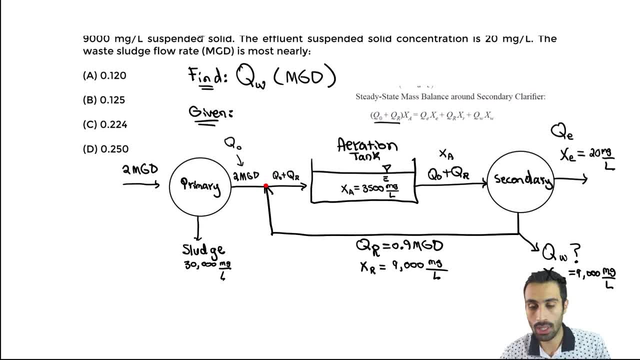 So this is our X E that comes out, Which has a corresponding Q E, and we'll look into that. Then we have QR. So QR comes out and know it's going to be this one, and we have X R at this concentration, suspended solids. 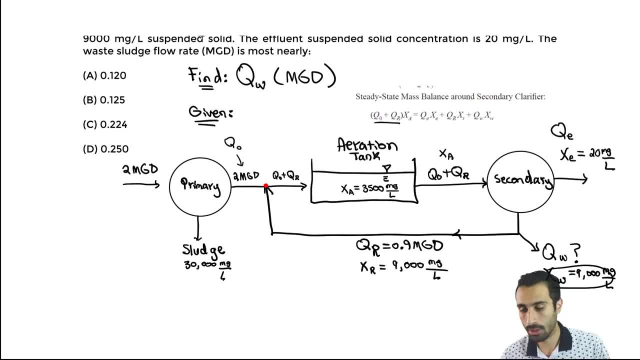 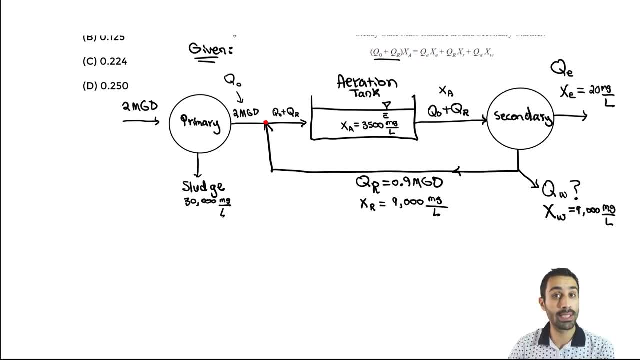 Then we have Q- W, which is what we want to find. Then we have X- W. that comes out. the secondary- Now let's start plugging stuff in So we know what comes out. the primary goes into the secondary treatment, which is going to be Q naught. 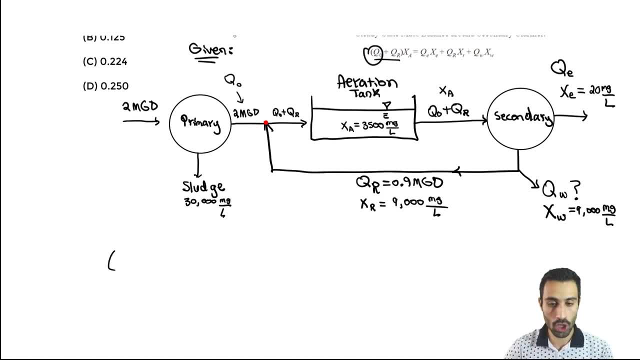 It's the 2 MGD, So we put that For the Q naught. So we put 2 MGD and then we add QR. We're adding QR because, no, this is around again the secondary, So we have to add QR. Q naught plus QR is what comes in. 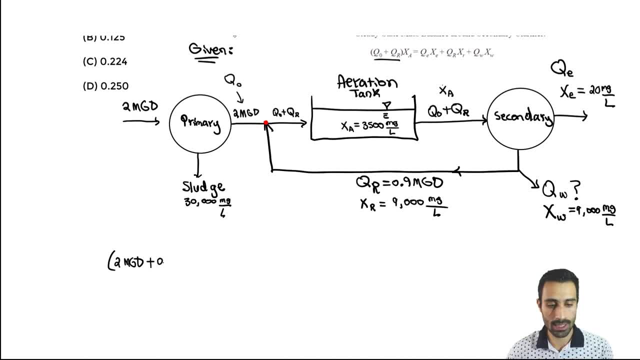 So we add that and that would be the 0.9 as given in MGD, million gallon per day. Then we multiply that by X, A, which is the MLS, MLSS, which is 3500.. In milligram per liter, Then we take that equal to. so this side is what comes in. 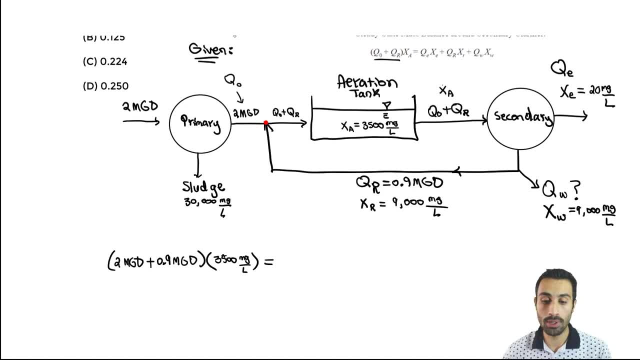 What comes out is going to be the Q E, X E, Q W, X, W, Q R, X, R, and that's what's denoted. So we know Q E is going to be a value that we do not have, So let me keep it there. 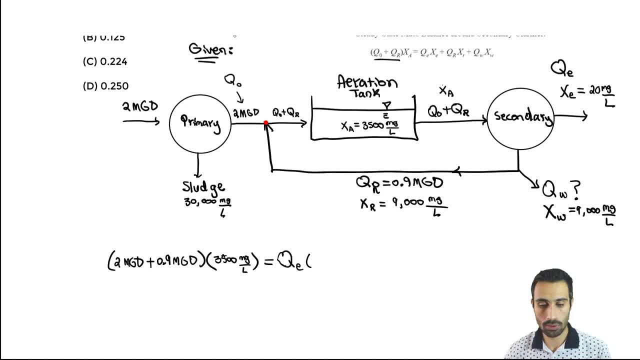 We can get that, though Then we would do X. E is going to be 20.. That's given Milligram per liter. Then we take that time plus QR, which is 0.9. And that would be MGD. everything in this case is MGD, milligram per liter. 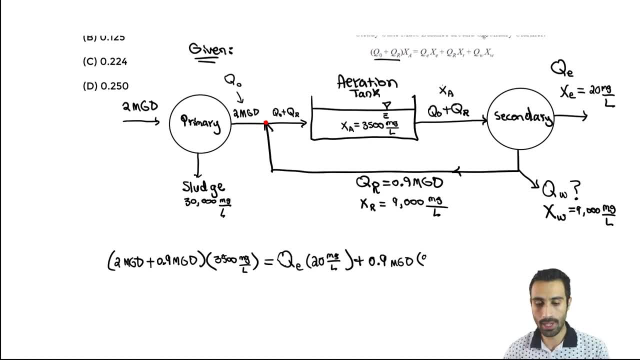 So that's QR. Then we do X R is going to be the 9000 milligram per liter. Then we do plus the Q W is going to be actually what we want to find. We don't know that. that's the goal to find. then X W is going to be 9000. 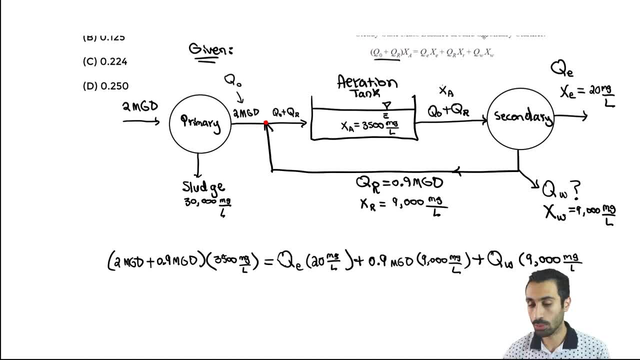 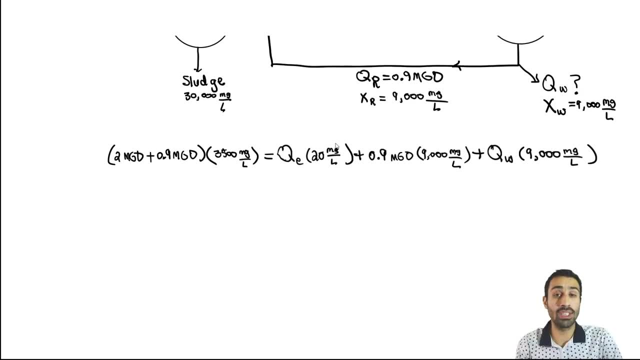 Milligram per liter. as we said always, X W is the same as X R. So now the problem we face is we have one equation, two unknowns, So we can't really do much with it. But there's something we can do. We can actually isolate that secondary clarifier. 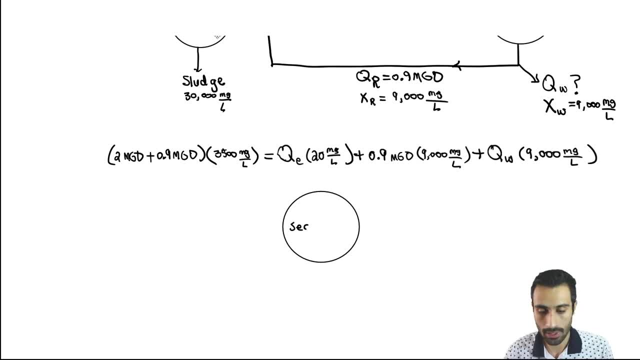 Let me denote this: for us, This is the secondary Secondary and if we look very close at this, we know we have something that comes out Q E- I'll just focus on the floor rates- and something that comes in which will be the Q naught plus. 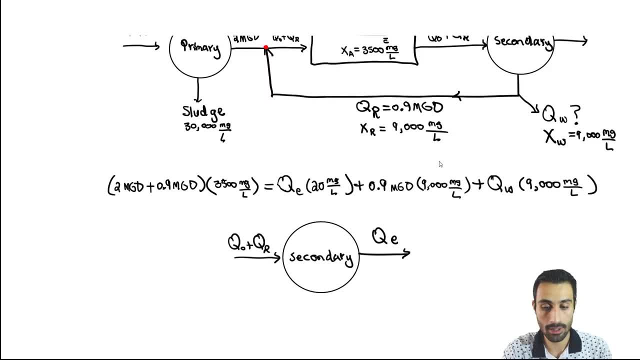 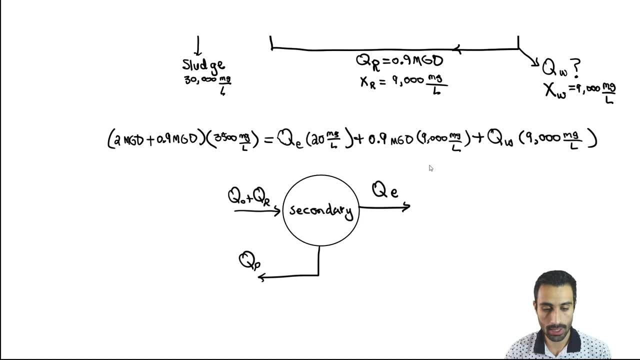 QR as we denote it here in secondary. Then we know stuff comes out of it down as well. So we have the QR that gets recycled, and we do have the Q W as well. So these are separate. We cannot combine these. So now, from this, what I'm going to show you is do a. 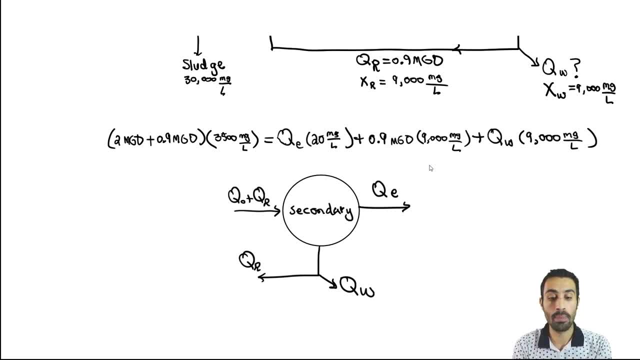 Mass balance or, in this case, continuity about the secondary in terms of floor rate. So we can say: whatever comes in has to come out. What comes in, what comes in is Q naught plus QR. This comes in right, then what comes out is everything else. 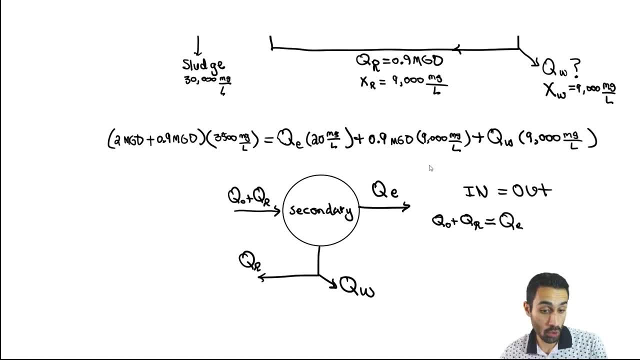 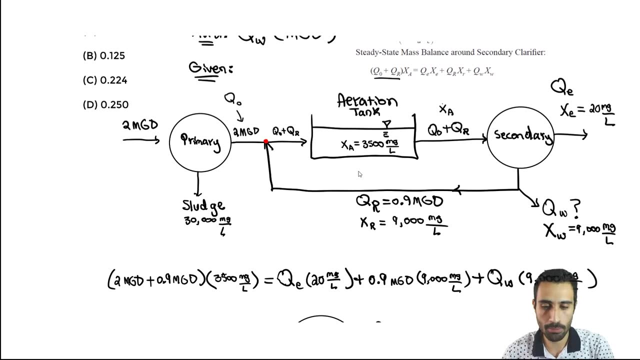 It's Q E. Let me denote that it's going to be QR and Q W plus QR plus Q W, and notice what happens with QR: They cancel. They're the same on both sides of the equation: equal sign. They would cancel, and that makes sense logically, because it comes in and it's just going to be recycled. 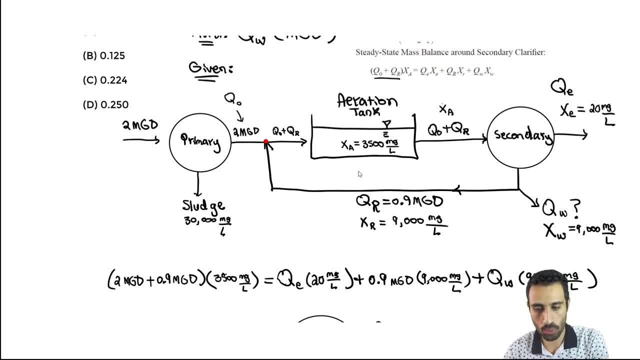 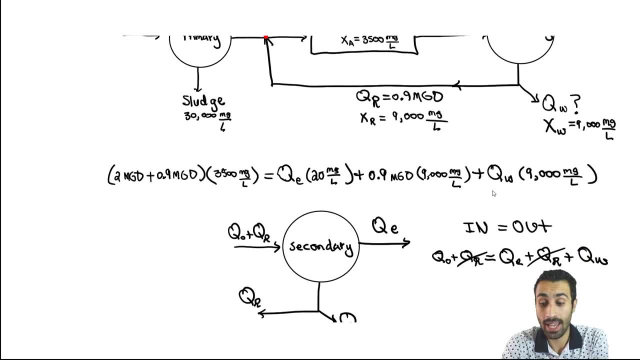 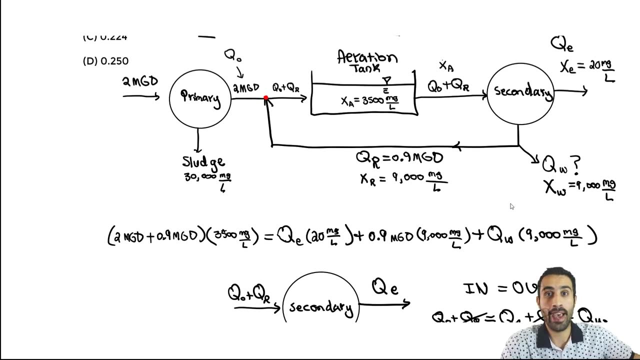 It's not like a floor rate that actually gets wasted like this. It's going to come in and just go in a loop that actually cancels. It doesn't do anything really for that secondary clarifier. We do recycle it into the aeration tank, though, to give it that activated sludge or that fresh. 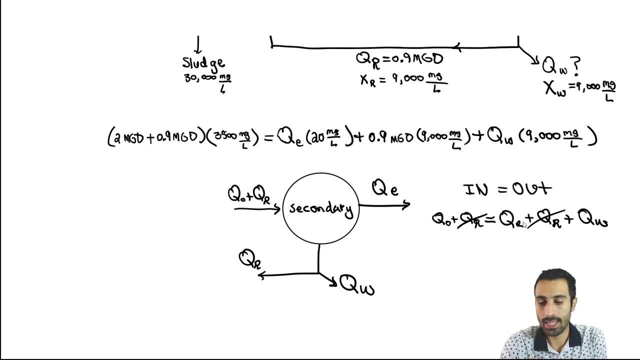 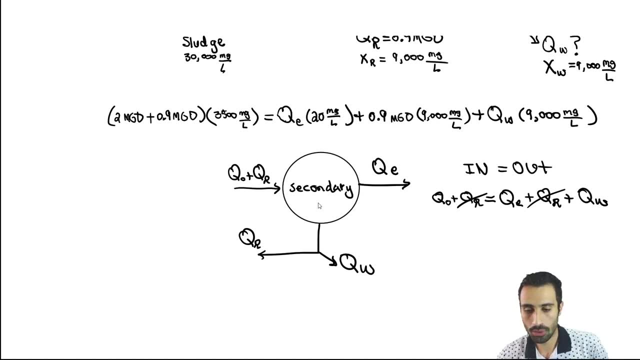 Sludge in that aeration tank. but we know that actually cancels when we look at this. So QR cancel. then we have Q naught is going to equal to this. So Q naught equals to Q E Plus Q W, and now we can isolate Q E to get Q naught minus Q W. 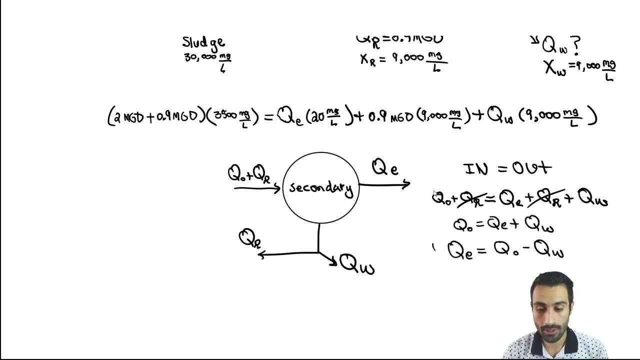 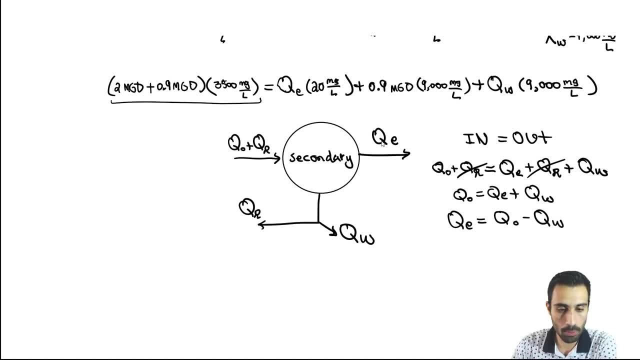 And why we did this is now we can take that Q E here and put it in here, and doing just that we can Start simplifying this. So let me simplify this portion first. So do the math with me. so we can take 2 plus 0.9 times 3500.. 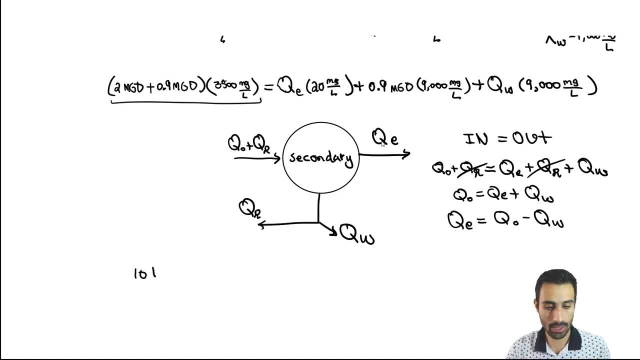 So we get 101.. 101, 50 that equals to. so we know Q E is going to be this part. So we did that and got that from a mass balance around a continuity balance around the secondary. So that would be Q naught minus Q W. 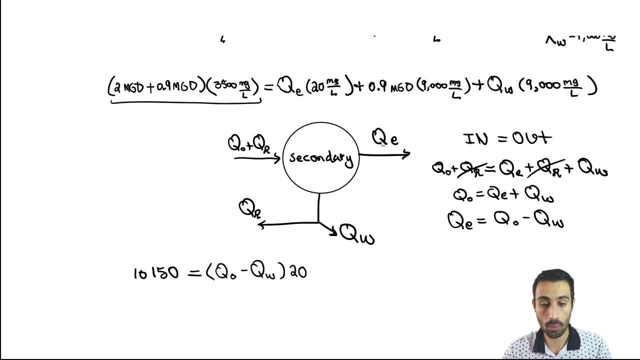 And that is multiplied by the 20, which is going to be this portion, Then we do plus 0.9 times the 9000. we get 8100 for that one, then plus Q W, Q W times the 9000, so that will just keep it like that. 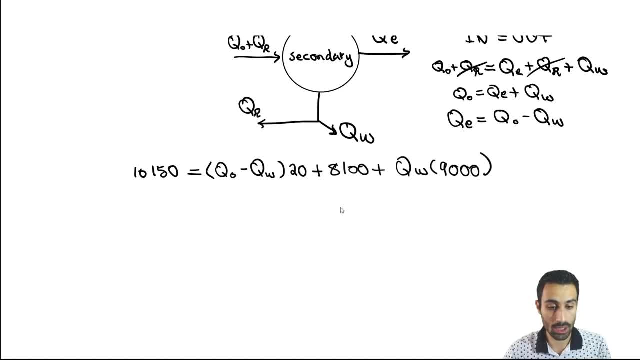 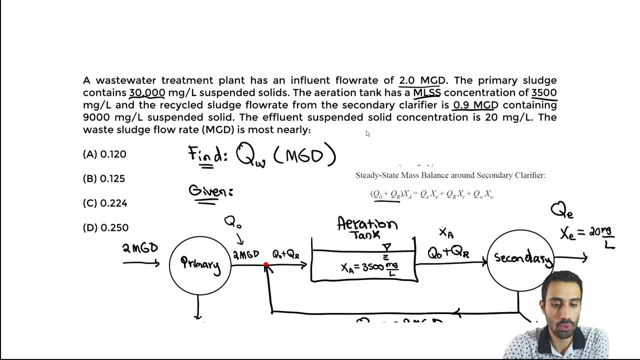 So now notice we have at this point we can actually plug in the Q naught, So that Q naught would be What comes in right. It says it's 2 and we denote it that as 2 MGD, So we just put 2 MGD for that one. 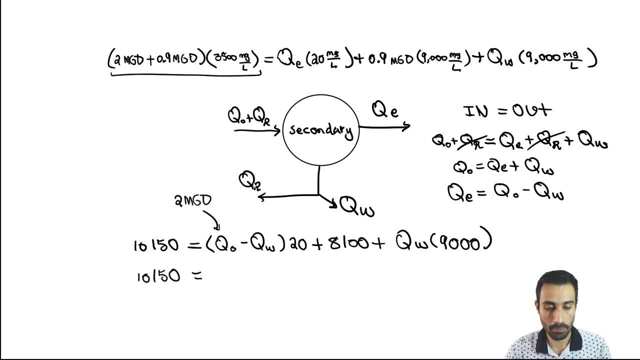 And we can reduce this. so it's going to be 101- 50.. So we put the 2 minus Q W is what we want to find. You remember that's the goal. times 20 plus 8100, plus we can put the 9000 in front just to make it look nice. times Q W. 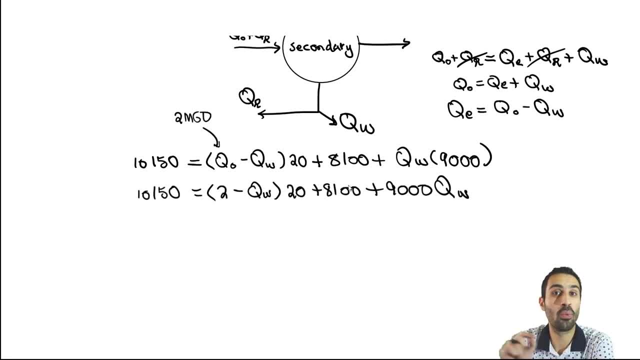 And now look at this. you have one equation, One unknown. we can find Q, W. So what you can do here is basically distribute the 20 and distribute the 20 to the 2. do that algebra, then combine like terms. It's going to be basic algebra.